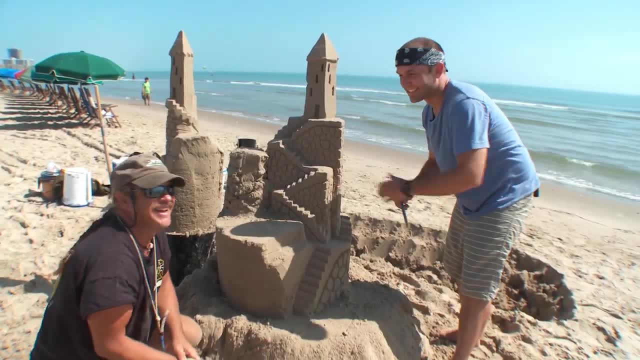 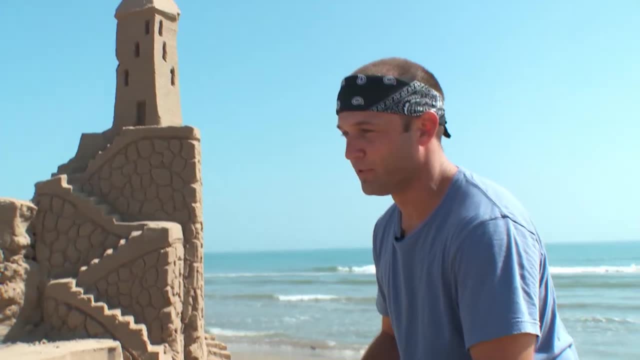 a little deeper, I'm busted. This is Dennis, the sand slave and master sandcastle artist. How's it going, Chad? Thanks for having us. Exactly, how do you start building something? This is obviously more than the dribble castles I've made. Well, it's basically the same way. 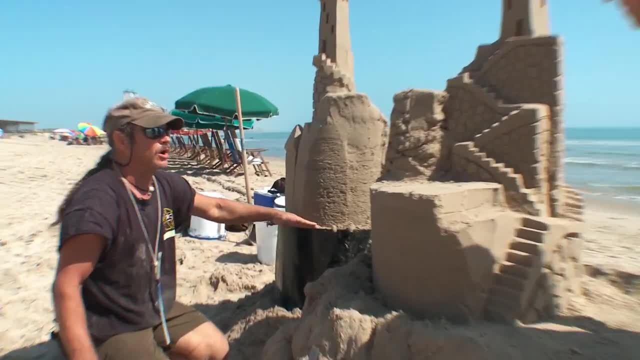 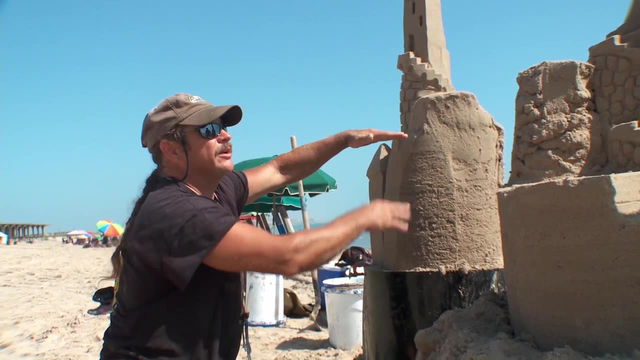 This part was done with a form. We put sand and water in this form here and then, when that's full of sand and water, we put another form on top, so it's like a wedding cake And at the very top here. 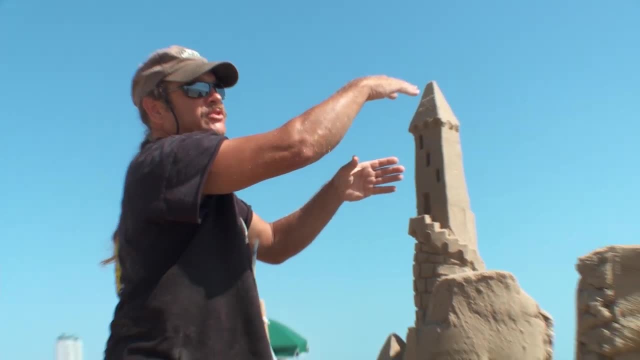 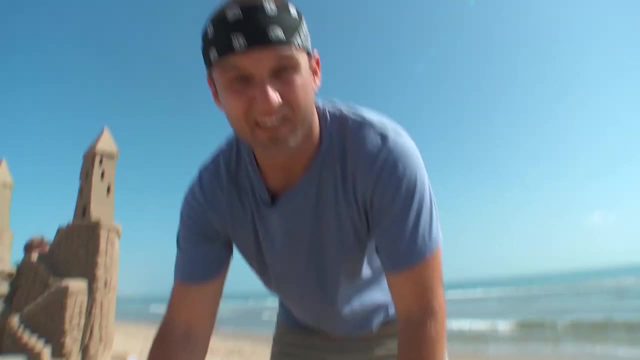 well, you can do a form where you hand stack. I'm going to show you hand stacking, sandcastling 101.. So let me go grab a bucket and bring it over there and I'll show you how to hand stack You. 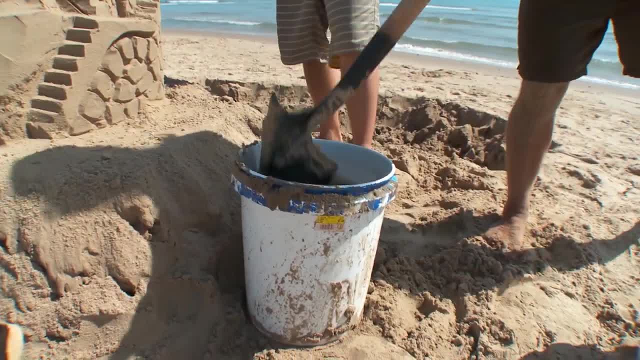 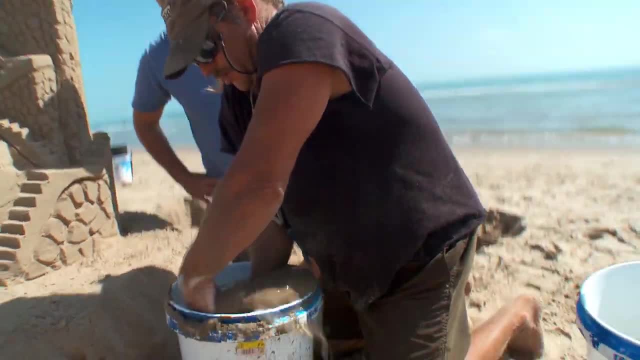 got to earn your keep here. Hey, I'll do whatever it takes to study under a true artist like Dennis. Texas is best sand slave, and today I'm getting my very own lesson. Oh, whoa, whoa, Pancake Boom One. 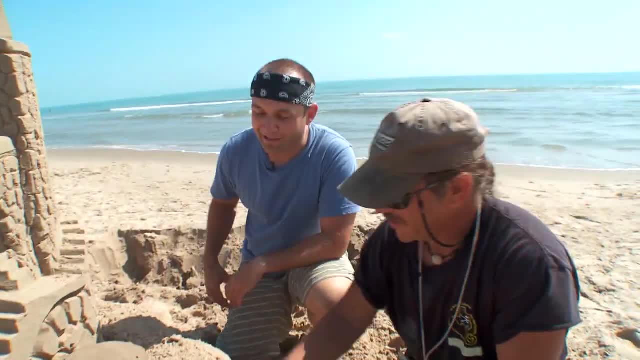 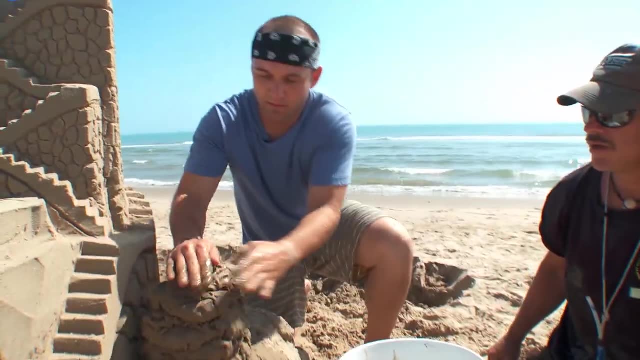 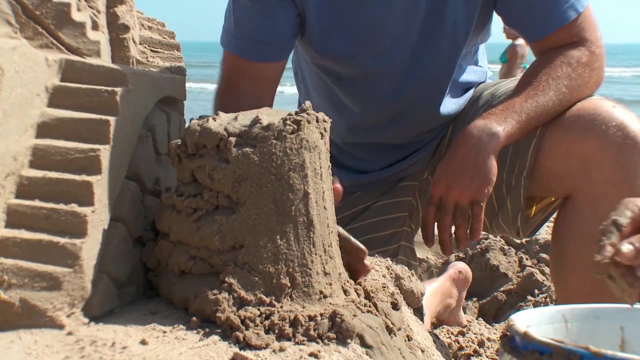 two, three, jiggle, stop, Ah. that's where I probably messed up, because I keep padding and the whole thing crumbles And it cracks. All right, There you go, Perfect. Ah, he said perfect, Nice, Perfect. So come in here like this, go all the way around, Straight up, straight up, or 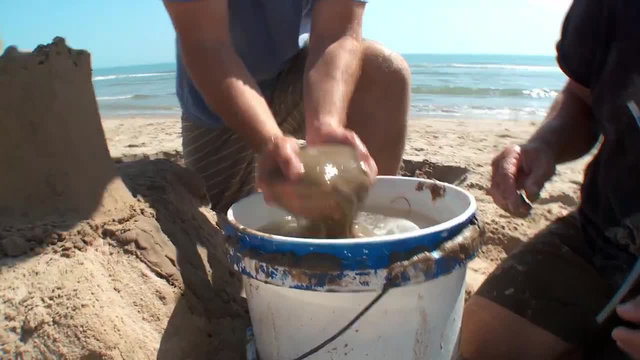 down. Am I looking for a straight line? Yeah, you are. I'm going to walk around. It fills in the cracks. We call this a kneeling. You guys have to have like the perfect sand here at South Padre to do this. 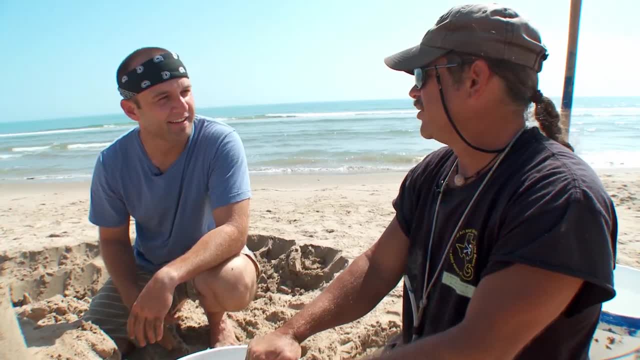 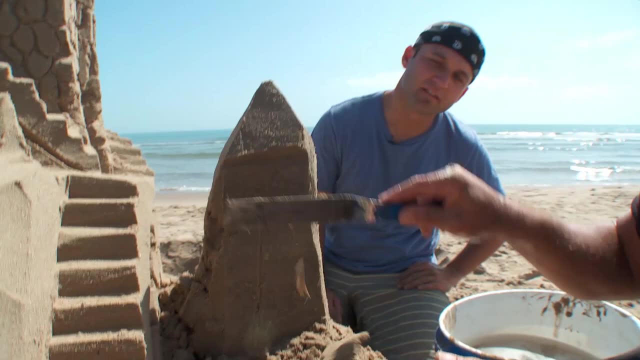 We have. this is probably the perfect place, because we can do this 365 days a year. We have the sun in the right place as it rotates around. We have great sand. This is your art form. Ah yeah, It's a perishable art. We'll see it today and it'll be gone tomorrow. 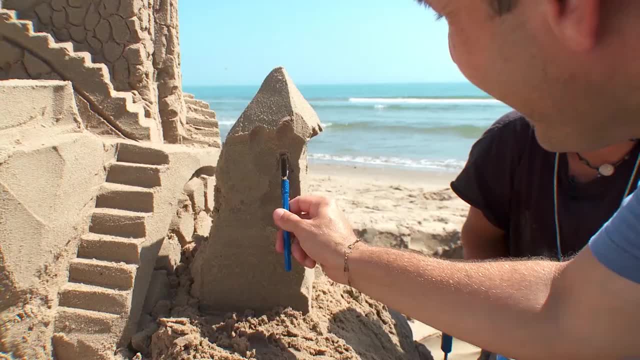 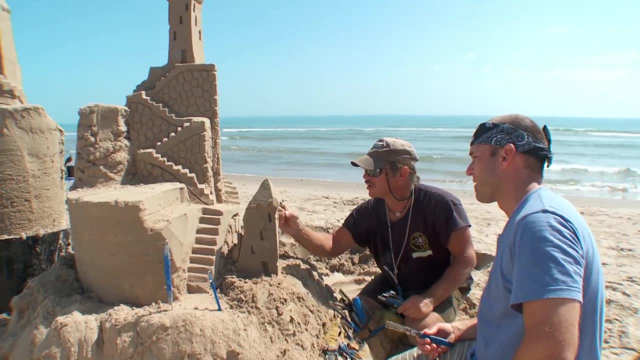 That's a lot of love and effort that goes into something that's just going to wash away, but obviously gratifying because we have students of all ages and we have the little kids, the grandparents- Cool- And they all work together on it. 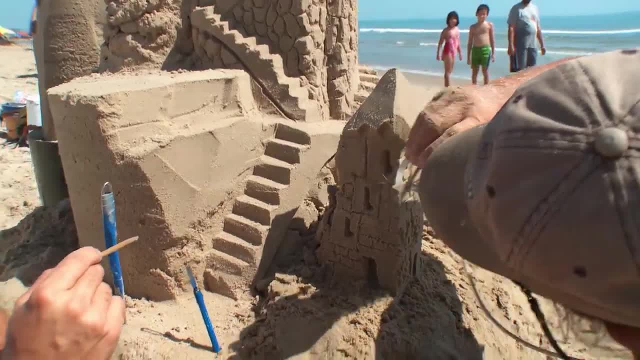 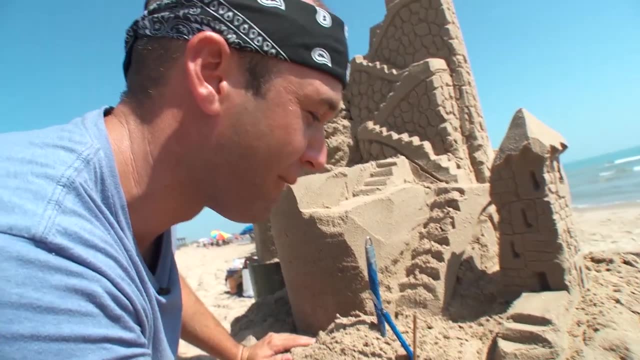 This is kind of rocking my Sandcastle world: the fact that you build something that looks nothing like what you want it to look like and then carve it away. It just feels natural to me. I feel like I'm finding some sort of calling. 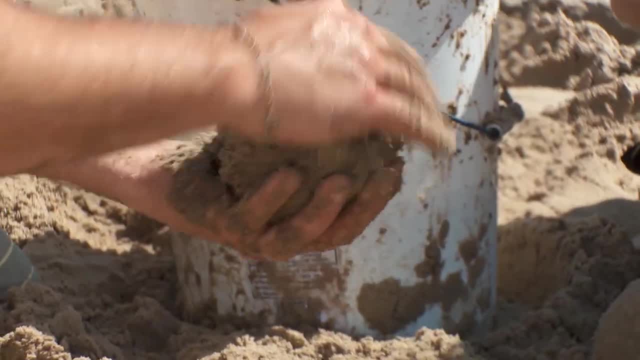 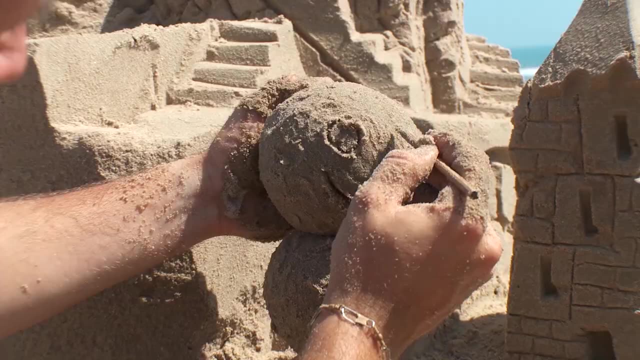 South Padre Beach is also the only place to build an authentic Texas snowball and snowman. Can you believe sand can do that? Amazing, I know, but it only gets better. We're going to build an arch, An arch Between here and here. 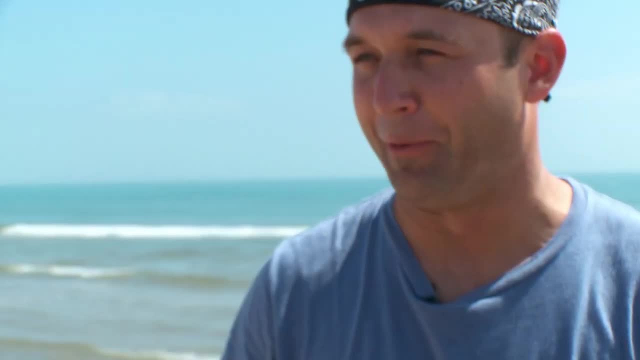 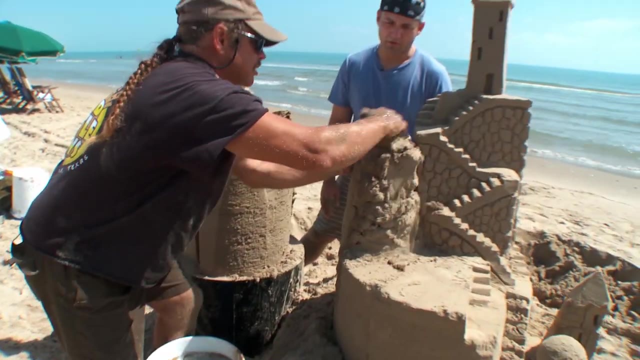 An arch. I don't think sand was ever meant to be an arch form. This is insane. We're going to start building across like this: Okay, So you can take your hands and as we go, I'm going to build over top of your hands. 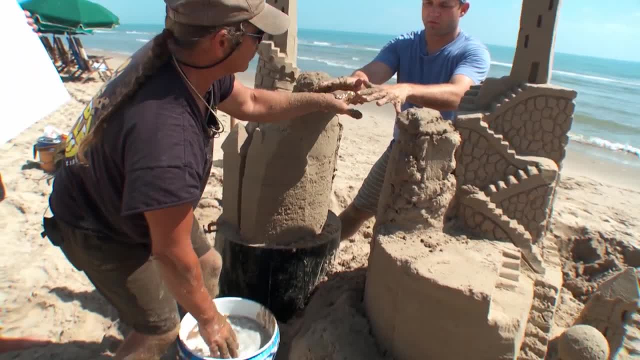 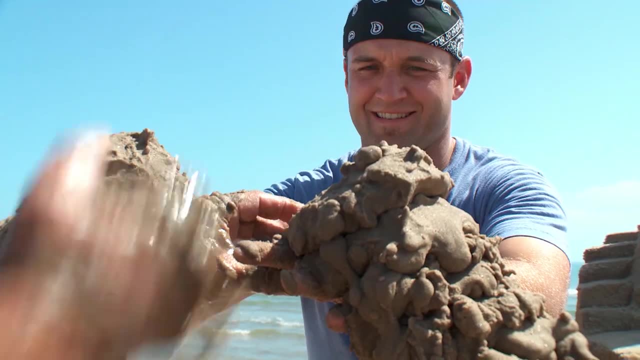 and you're going to keep the arches or the two towers from falling into each other. Okay, Spread the fingers out, But you've been doing good. Hold steady. Yep, This is a wide span. This is awesome. The Romans were really famous for doing their arches. 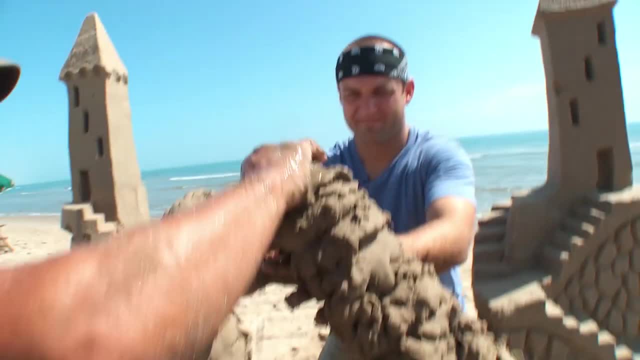 but we're going to be famous right now for making ours. You told me when, All right Now, slowly wiggle our fingers and pull them out. The moment of truth. Ta-da, Whoa, Whoa, My mind is blown. 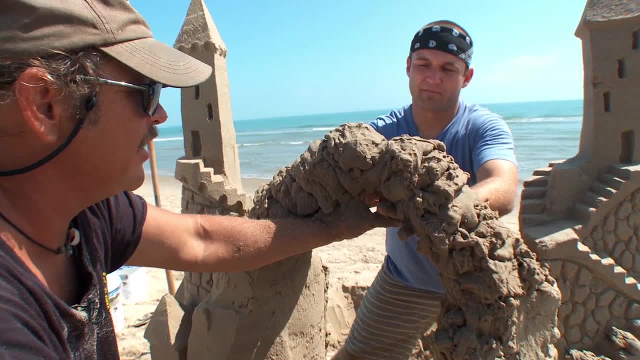 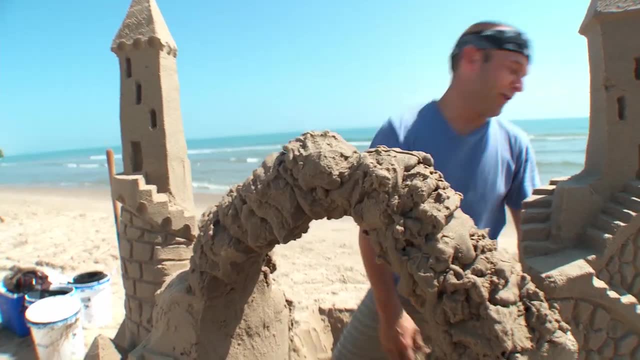 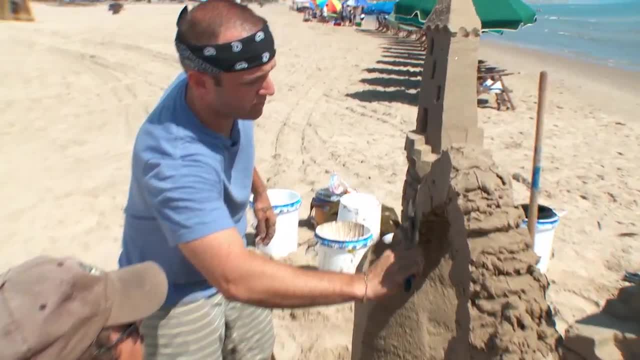 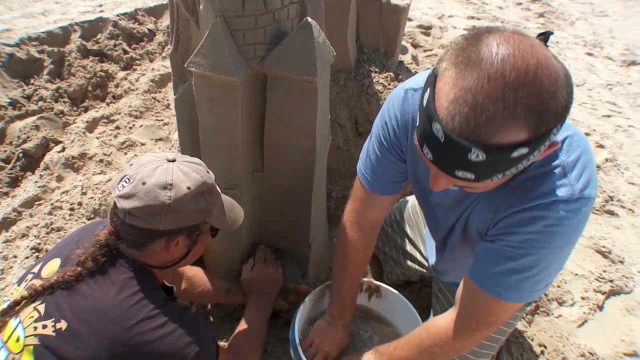 It's like destructive and creative at the same time, which I'm all in. It's got to be a blast for families to get out here, get muddy together. I had one where the mom said I can't believe my three sons are working together. 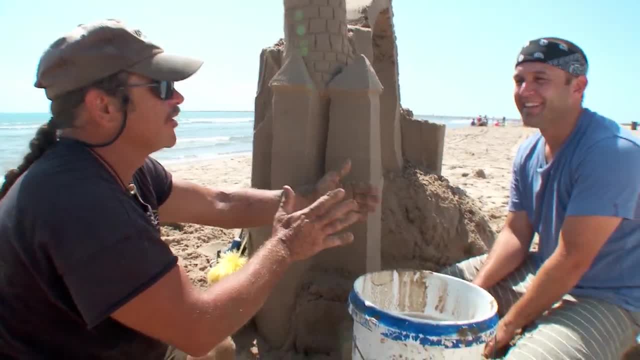 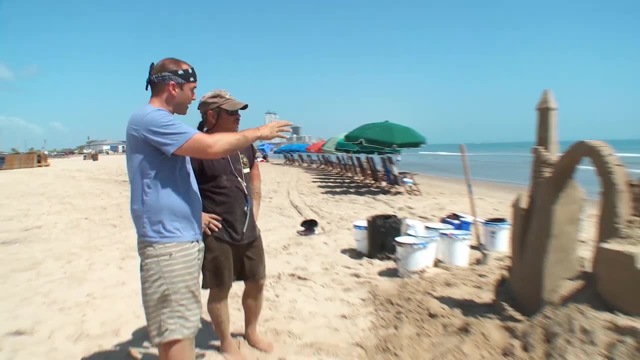 And there's a picture of them all, three of them together, working on the same part of the sandcastle. together Sandcastles, bringing families together, There we go. Millions of pieces of sand, millions of possibilities, but only one proper name. 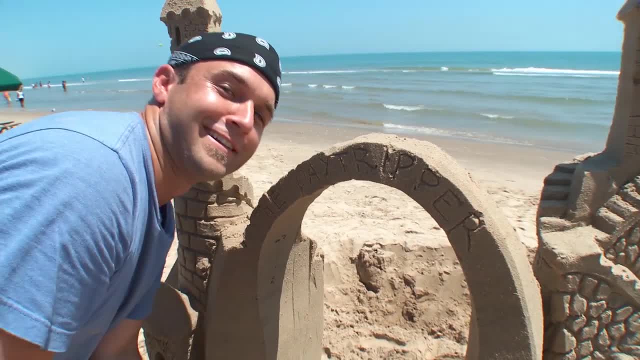 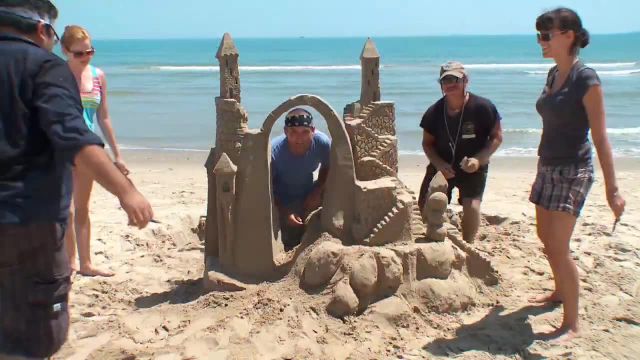 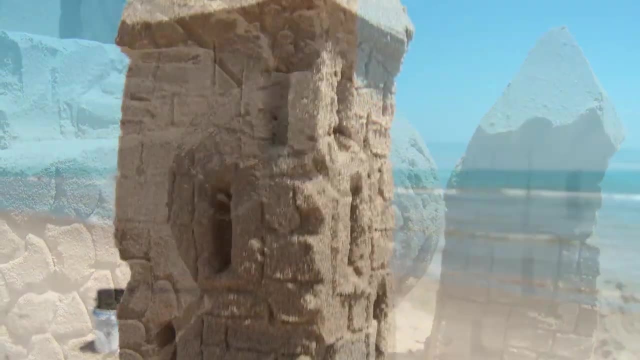 The Day Tripper Castle For our monumental team effort, A monument that will stand for but a brief moment before it fades back into the sea. It's sort of like life: The sea and the sand, and the waves and tides of change. 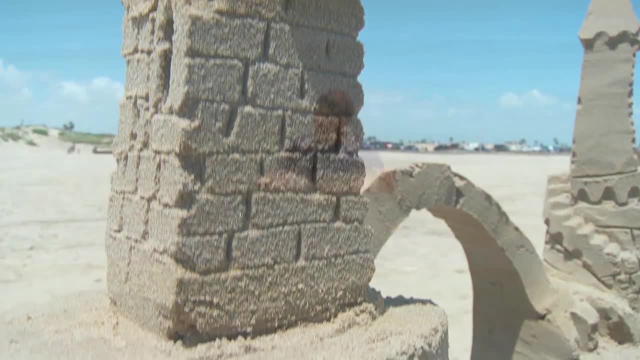 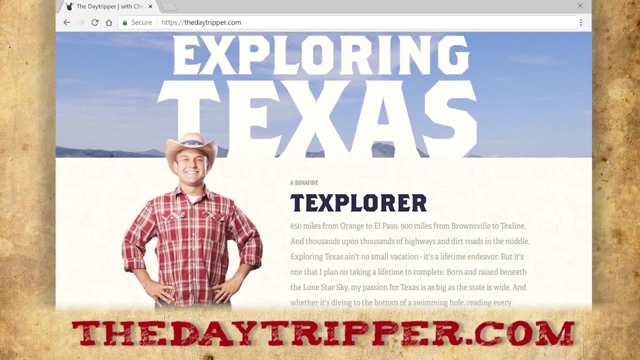 Yeah, I'm sure there's some deep analogy to make here, but it is very hard to think with all this sand in my pants. Ah well, I missed it To see the full episode or to get info about how to visit this spot.